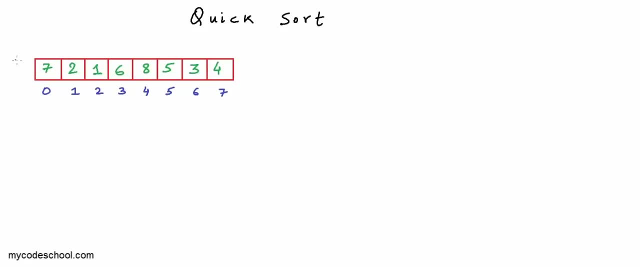 given to us in the form of a list of integers. Let's say, we have a list of integers given to us in the form of an array, something like this. I will name this array A, and we want to rearrange this list in increasing order of the value of integers. Now in quick sort. 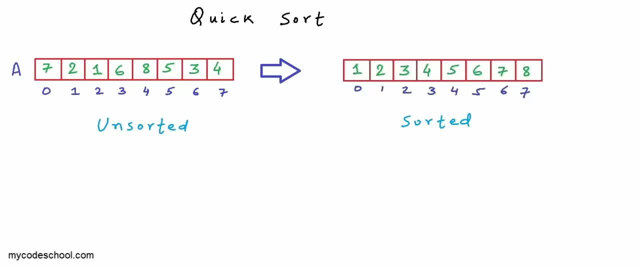 what we do is we first select one of the elements from the list, and this can be any element In this example here. let's say we select number 4. Now we call this selected number pivot, And now first we rearrange the list such that all the elements lesser than the pivot are towards. 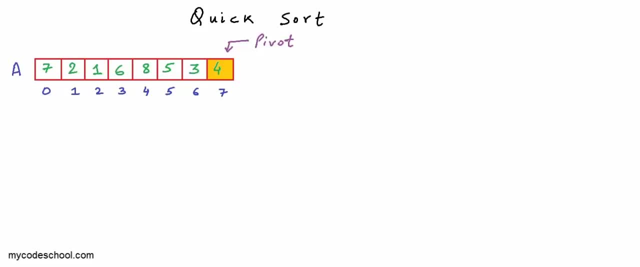 the left of it and all the elements greater than the pivot are towards the right of it, something like this: Let's call this whole process partitioning of a list. So let's say partition is a process in which we select a pivot and rearrange the list such that all 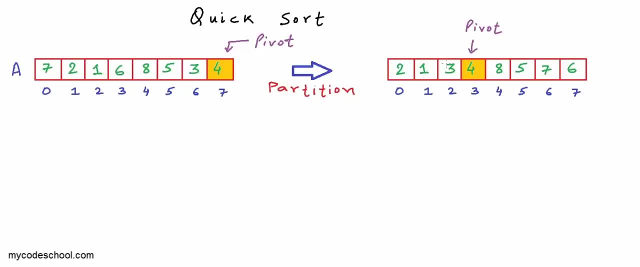 the elements lesser than the pivot are towards the left and all the elements greater than the pivot are towards the right. There can be more than one possible arrangements in which elements lesser than the pivot will be towards the left and elements greater than the pivot will be towards the right. For example, 2, 1 and 3 are lesser than the pivot In this. 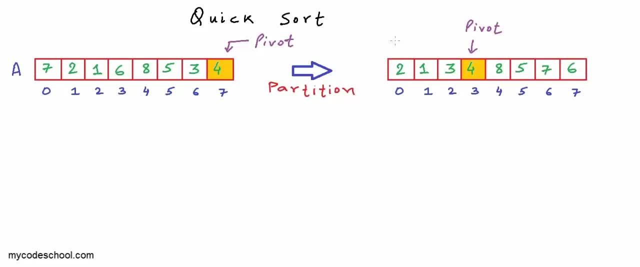 example, we could have had them in order 3, 2, 1, or 1, 2, 3.. It doesn't really matter, We can have any one such arrangement. The only requirement is that all the elements lesser than the pivot should be towards the left, and all the elements greater than the 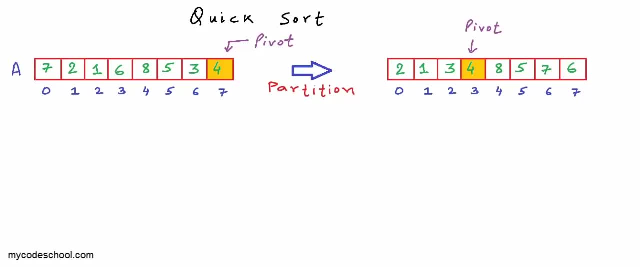 pivot should be towards the right. We have an efficient in-place algorithm to partition a list like this. We can do so in constant amount of extra memory using only some temporary variables. We will come back to the partitioning logic, But let's first think about this Once. 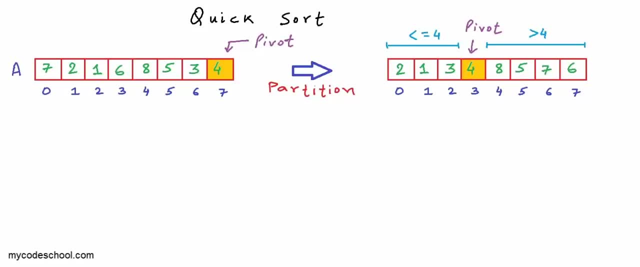 we have partitioned the array like this. we can break this problem into two sub-problems And the two sub-problems will be the following: We have a list of two sub-problems. We will will be sorting the segment of the array to the left of the pivot and sorting the segment. 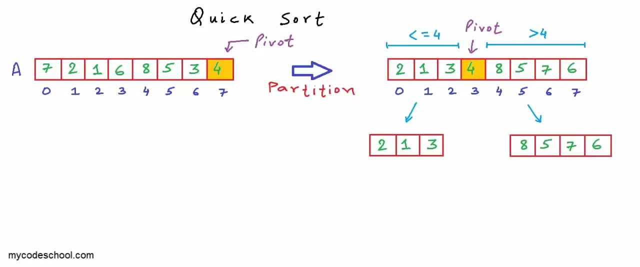 of the array to the right of the pivot. And this time, unlike merge sort, we do not need to create auxiliary arrays, entirely new arrays, and copy the elements into these new arrays. we can work on the same array, It's just that we will have to keep track of the start and 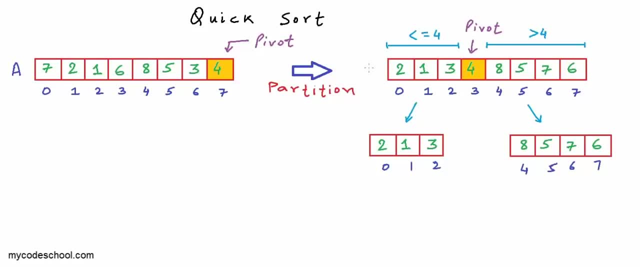 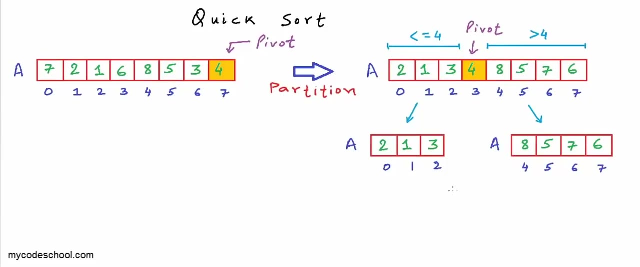 end index of these segments. So if this is array A from index zero to seven, this is segment of array A from index zero till two And this is segment of array A from index four till seven. we will come back to why we do not need to create auxiliary arrays. 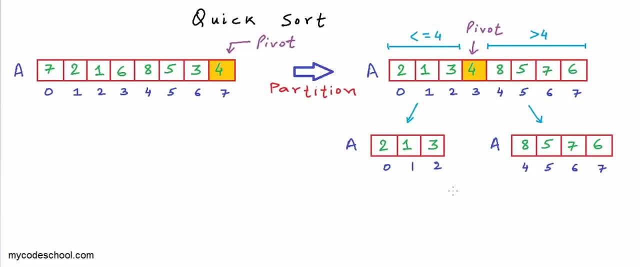 and why we can work on the same array just marking the start and end of a segment. Let's first try to understand the core logic. So far, we understand that once a list has been partitioned, then we have two sub problems to solve: sorting the 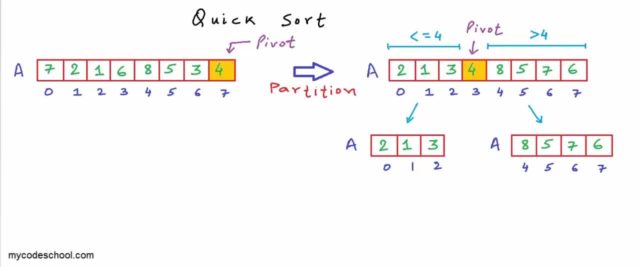 list left of the pivot and then sorting the list right of the pivot, sorting the sub list left of the pivot and sorting the sub list right of the pivot. But now how do we sort these two sub lists that we have created? we can apply the partitioning logic once again. 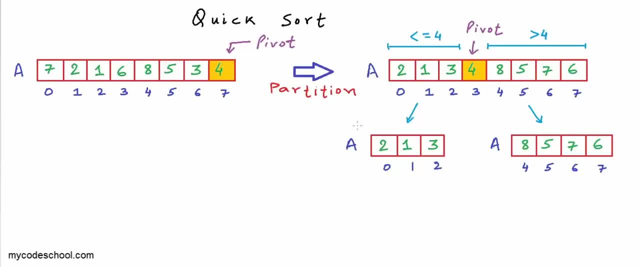 and break the problem even further. Let's say, first we want to work on this left sub list, So pick up the pivot, and then we rearrange this sub list such that all the elements lesser than the pivot are towards left. three is the largest in this sub list, So this arrangement. 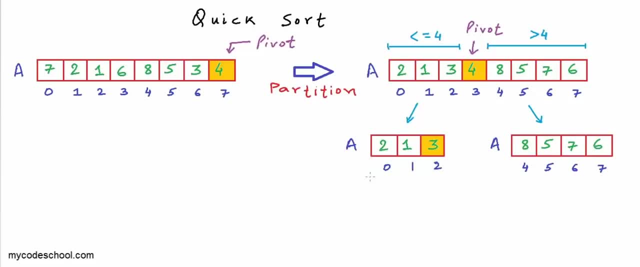 is actually satisfying the condition And this problem will actually have only one sub problem. Now we need to work on segment of the array from zero till one, because there has to be a deterministic logic of picking up the pivot. Let's say we always pick the. 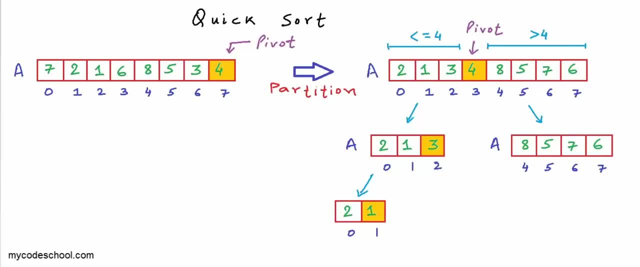 right most element in the sub list as pivot. So for this segment, from zero till one, we will pick one as pivot And this sub list will be rearranged like this And we will have one sub problem to solve. So we are going on in a recursion, we are breaking the 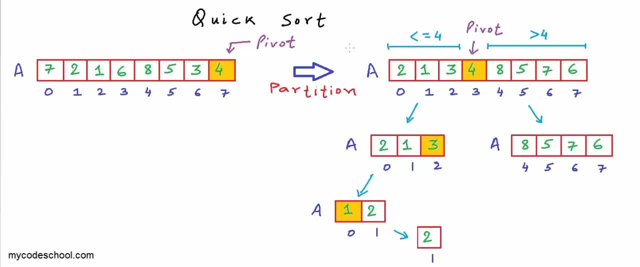 problem in self similar manner. And remember, all the rearrangement is happening in the original array, only in the original list, only In these segments that we are showing here are just snapshots of the original array. So at this stage we have 2,, 1 and 3 at 0,. 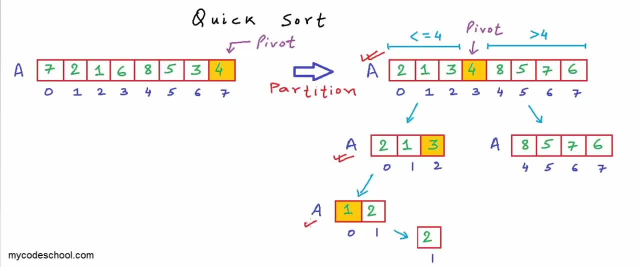 1 and 2 respectively in A, And when we go to this stage, after partition, 2 goes to index 1 and 1 comes to index 0. So when we are here, when our segment is only one element, the element at index 1, then the original array from index 0 till 2 is 1, 2 and 3 at. 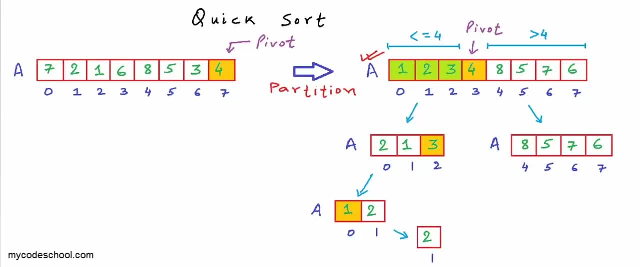 indices 0,, 1 and 2 respectively, And when we have only one element in a sublist or a segment, that segment is already sorted. we do not need to break the problem any further. So we need to stop our recursion at this stage. This will be the exit condition from. 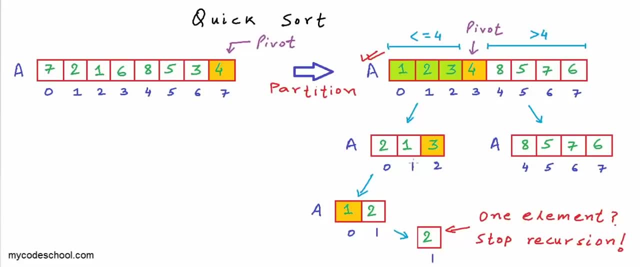 recursion, And at this stage the segment from 0 till index 2.. 2 is sorted And now we can go ahead and work on the segment from index 4 till 7.. Now let's first try to understand how we will do all of this programmatically. I will write a function named 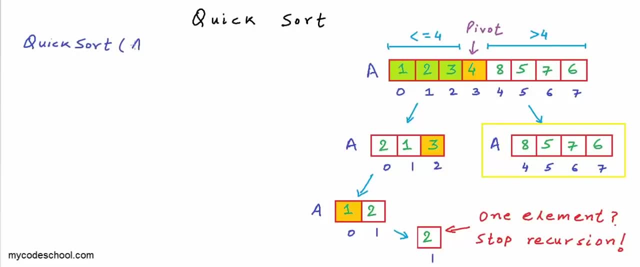 quick sort that will take as argument an array, a and start and end index of the segment that needs to be sorted. Now, why do we need start and end as argument? Because we do not want to create any auxiliary array, any new array. What we want to do is we want to use the same. 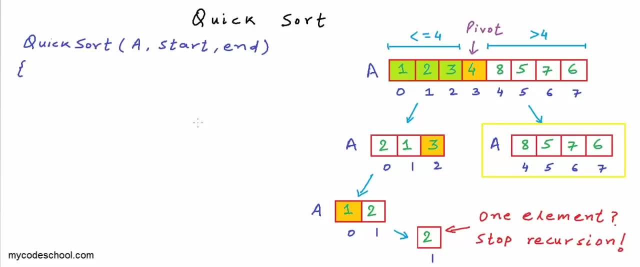 array. We want to keep on passing the same array and we just want to mark the boundaries of the segment that we want to work upon. Initially we will call the quick sort function, passing it start index 0 and end index length minus 1.. So we will pass the whole array. 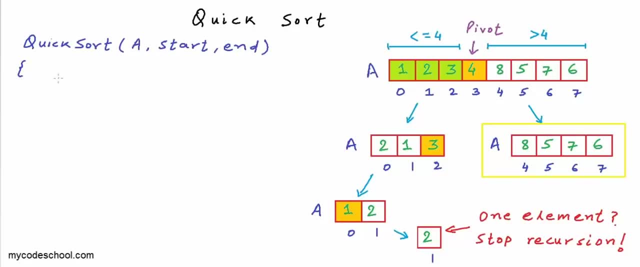 Things will be clear when I'll write the body of this function Now. in this function, first we will make a call to partition, the array And to partition also we will pass the array, the start index and the end index to tell that you need to work only on this segment. Now this function: partition. 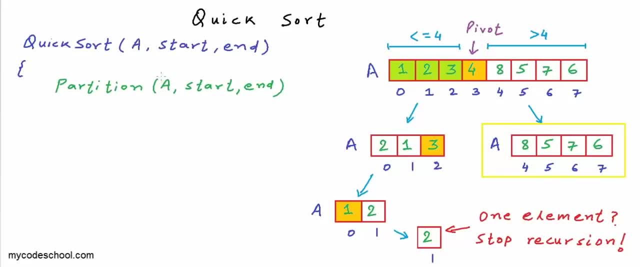 let's say, will rearrange the array such that will rearrange the segment of the array from start till end, such that there will be a pivot and all the elements left of the pivot will be lesser and all the elements right of the pivot or towards the higher indices of the pivot will be greater. 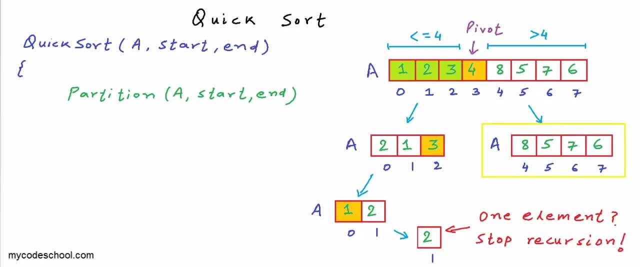 And let's say, this function will return the index of the pivot. after rearrangement, I will call it p index for partition index. Now, once we have rearranged a segment in this process- partition- and got the partition index, the index of the pivot, then we can make two recursive calls. 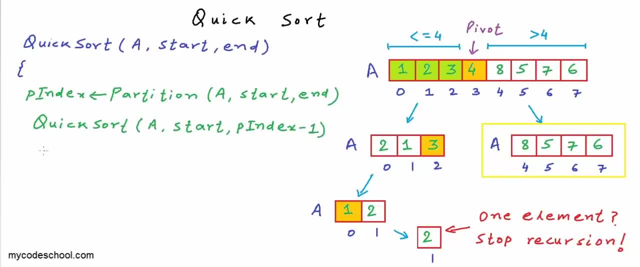 one to sort the segment left of the partition index and another to sort the segment right or towards the higher index, higher indices of partition index. So first call is for segment start till partition index minus 1 and another call is for segment starting, partition index plus 1 till end. There is only one thing remaining here. 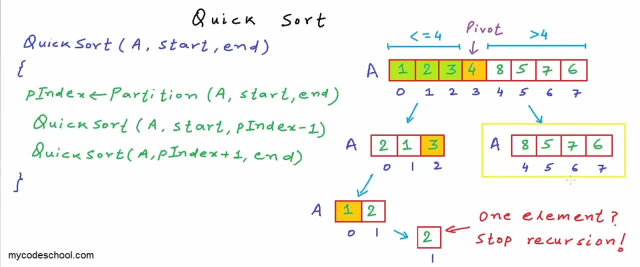 now. we do not want to go into the recursion infinitely, so we must write a base condition or exit condition in our function here, As we had seen, we can exit if a segment is having only one element. so we can write something like this: if start of the segment. 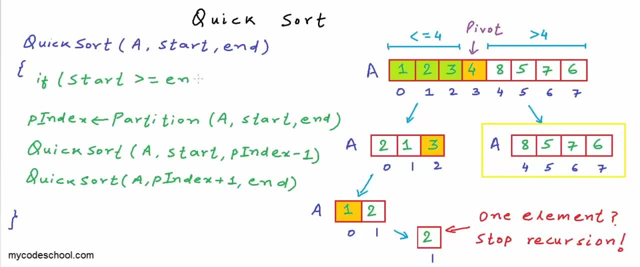 is greater than or equal to end, then we can return, which will mean exiting the function. Why start greater than or equal to end and not just start equal, equal end? Well, start greater than or equal to end will take care of two things if the segment is invalid. 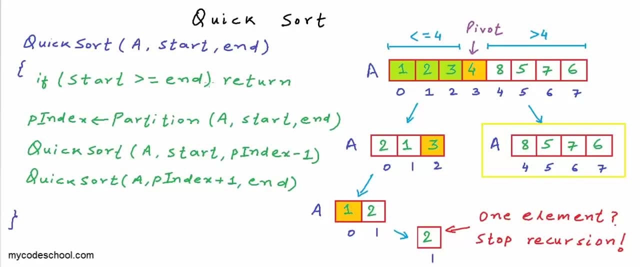 then also we will exit. and if segment will have only one element, then also we will exit. Sometimes we will not have a valid segment in the left or in the right, like here for this segment. from index 0 till 1 there is no segment left to the pivot, but still we will make. 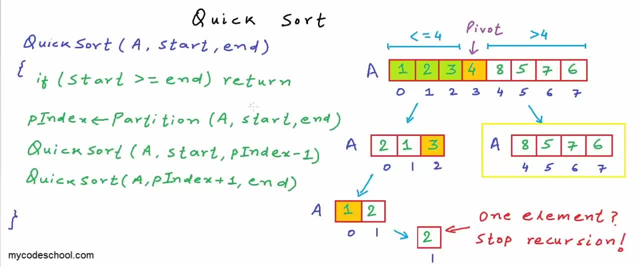 a recursive call to quick sort, We need to gracefully exit. in that case, We can also write something like this: do this whole partitioning only if start is strictly less than end, and this will also mean the same thing. We will come back to partitioning logic, which is the core of this algorithm. 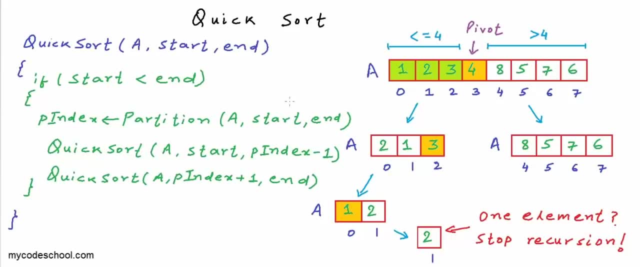 but first I'll quickly simulate a run of quick sort on this example array here. First we will make a call to quick sort passing it array start index 0 and end index 7.. Now start is less than end, 0 is less than 7, so partition function will be called. 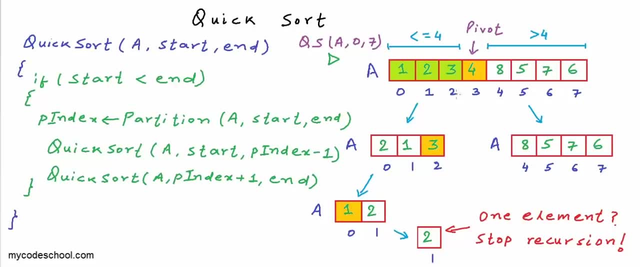 and after partition, partition index will be 3, so this quick sort call will make another quick sort call with start index 0 and end index 2.. Whenever a function makes another call, the execution of that particular function call is paused. The machine says that: hey, I'll come back to you once I'm done. 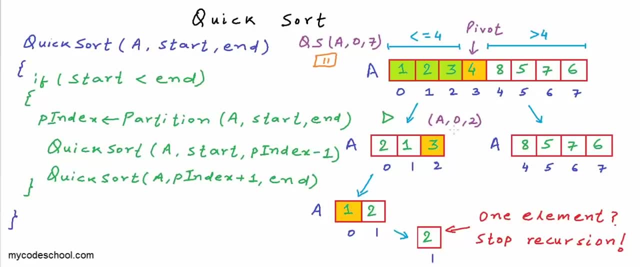 Once I have finished this another call, I'll simply write q here as shortcut for quick sort. Now, once again, 0 is less than 2, so we will partition and this guy q will first make a call to q. The state of execution of this call. 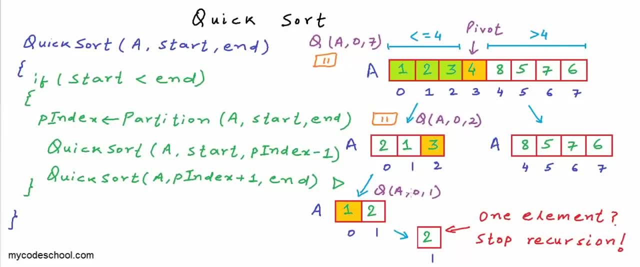 will be paused. We will go to q. 0 once again is less than 1, so partition will run. We are already showing the partitioned segment here, and first a call will be made to q and partition index here is 0, so we will make a call like this: 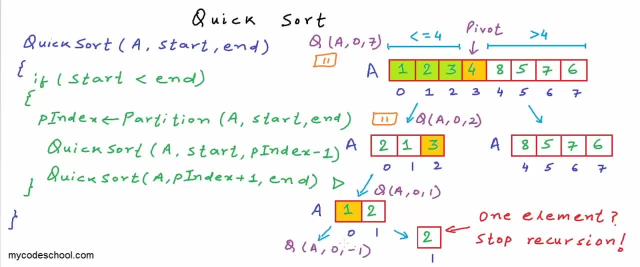 Now start equals 0 and end equals minus 1 is an invalid segment, but our code is taking care of it. We will not go inside the if condition here for this particular call, and this particular call will simply finish and exit. So this guy will simply return without doing anything. 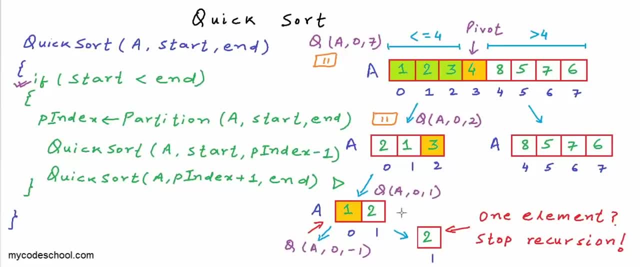 The control will return back to q, and now this guy will make another recursive call to q. Now, once again, for this guy, start less than end condition will be false. so this guy will not partition, It will simply return. and now q will return, and now q will make another call. 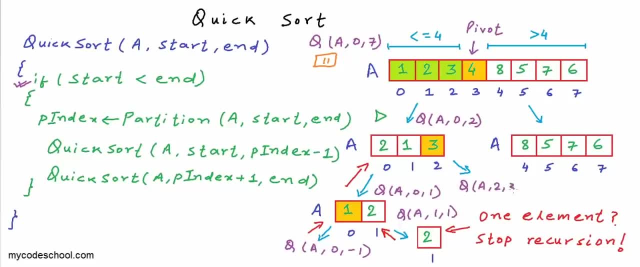 to q. Sorry, a32, it has to be p index plus 1 till end. Once again, this is an invalid segment, so this guy will simply return and now q will return. q will resume And now q will make a call for the segment right of the pivot. 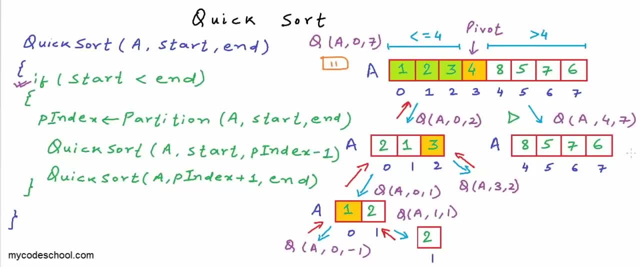 A call like q will be made. 4 is less than 7.. So first partition will happen. After partition, pivot will be 5.. Now q will make call to. it will first make a call like q, start 4, end 4, which will simply return because we have 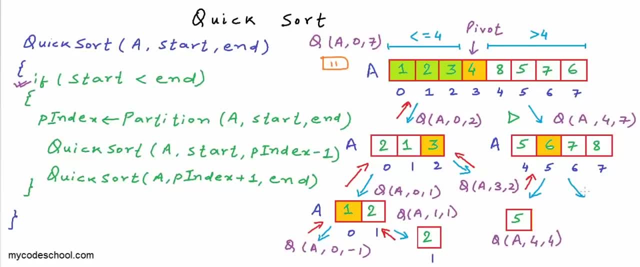 only one element in the segment, Then it will make another call for segment from 6 to 7.. This guy will again make two calls, One for an invalid segment. The right one will be for invalid segment and one for the left one. First it will make a call for the left one. 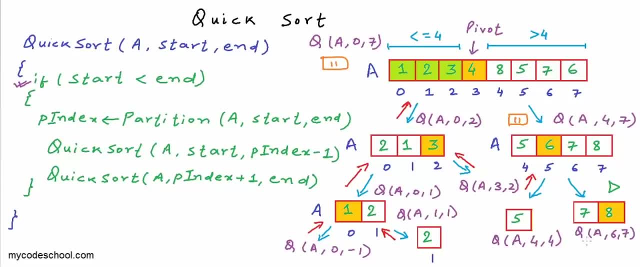 The left, one will have one element in the segment, so that will also simply return. So finally, with all these calls, our list in all will be sorted. once the right sub list is also sorted, The list itself, the overall list, will also be sorted. So this is how things will happen. This is how things will execute for this. 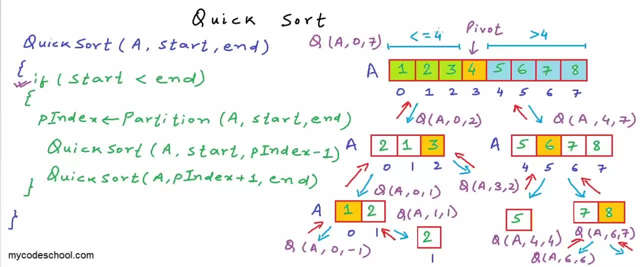 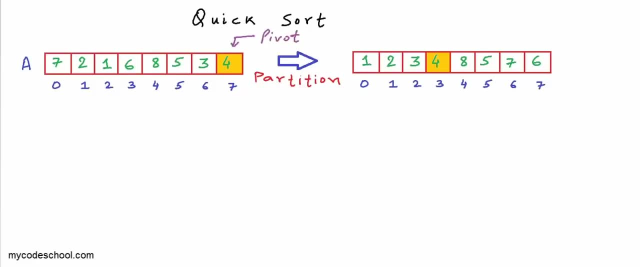 recursive function: quick sort. Now let's talk about the partitioning logic. Basically, we want to solve this problem. We want to select a pivot and we want to rearrange a list such that all the elements lesser than the pivot are to the left of it and all the elements greater than the pivot are. 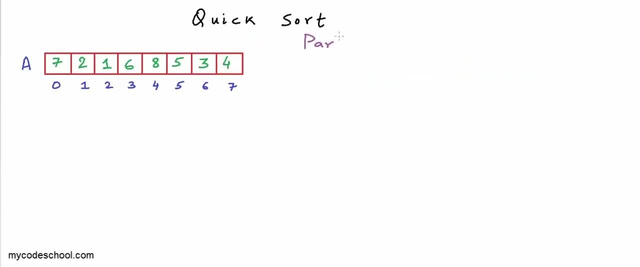 to the right of it. I want to write a function named partition that should take an array, The start index of the segment in the array that needs to be partitioned and the end index of the segment. This signature will make sure that we have a function to partition a segment of. 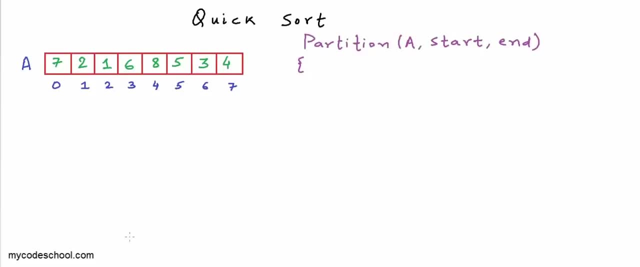 array a. You can pass the whole array to this function or you can pass a segment. You just need to pass the right values for start and end. Now in this function we first need to select the pivot, Let's say the right most element in the segment is selected as. 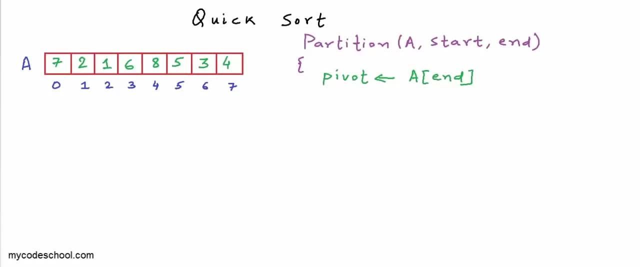 pivot. So pivot is always a end. If we pass this whole array, we will pass a. Start will be 0,, end will be 7. So pivot will be 4.. Now partition logic will be something like this: We will first take a variable named. 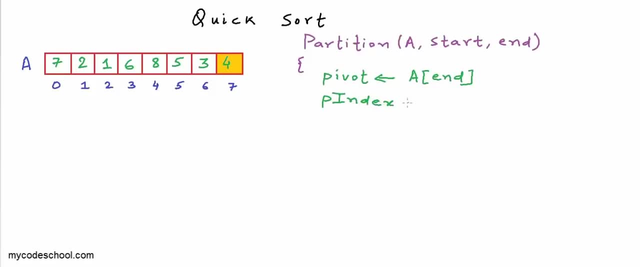 p index or partition index. I'm just writing shortcut p index for partition index and initially we will set it to start and now we will scan the whole list from start till end minus 1 and we will make sure that the elements lesser than the pivot are pushed to the left of partition index. 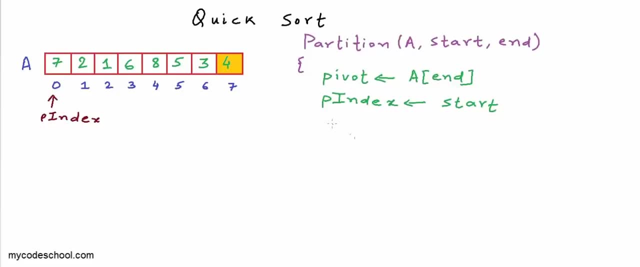 Partition index will be adjusted accordingly. So we will do something like this: We will run a loop from start till end minus 1, and if the element at that particular index is less than or equal to pivot, we will first swap that particular element with the element. 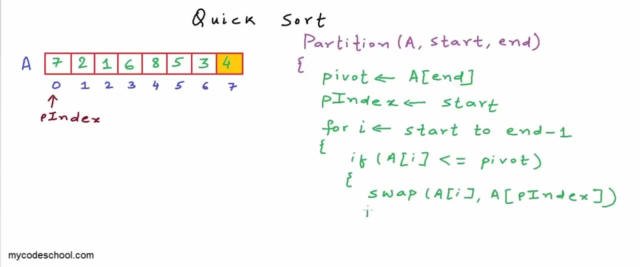 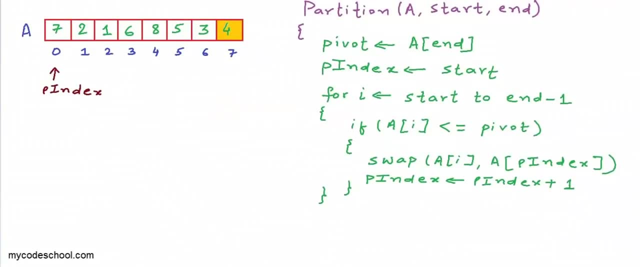 at partition index and then we will increment the partition index. With this much of code, let's quickly see what will happen if we will try to partition this array that we are showing in the left here. We will pass this array. Start index will be 0,. end index will be 7.. 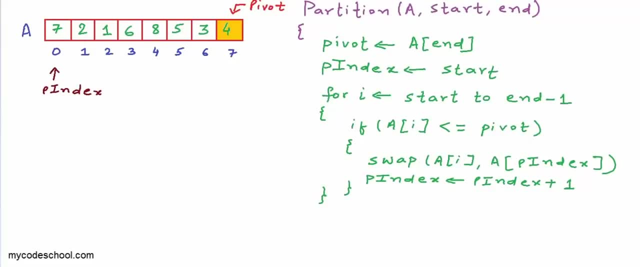 So 4 will be the pivot. p index will initially be 0. Now the idea is to push all the elements lesser than the pivot to the left of p index. We will start the for loop with: i equals 0. We will come to this conditional statement. 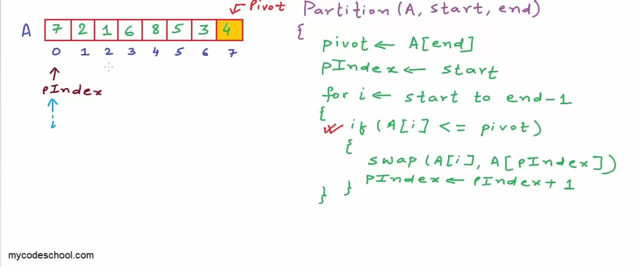 7 is not less than or equal to 4.. It is greater than 4.. So no swapping will happen. I will simply get incremented. Now a, i will be 2.. 2 is lesser than 4.. So we will swap the elements at index i and at index 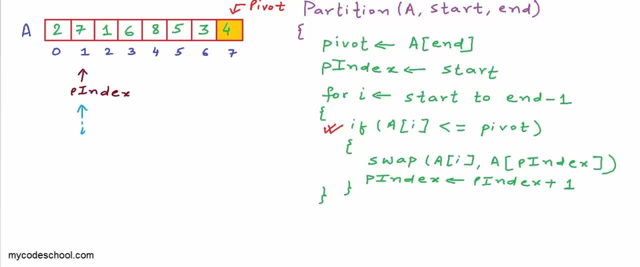 p index. and now p index will be incremented At any stage. all the elements to the left of partition index will be lesser than the pivot. Let's say we will show them in this blue color. Now i will be incremented, I will be 2.. 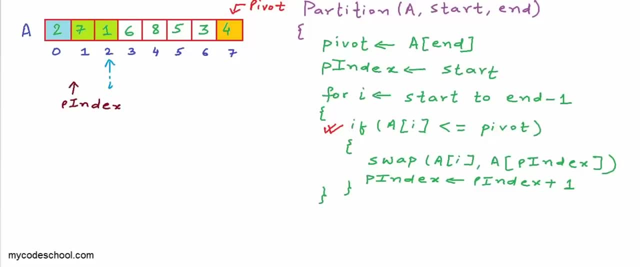 1, once again, is lesser than 4.. So we will swap these two elements, 7 and 1. Partition index will now be equal to 2 and i will be 3.. 6 is greater than 4. So we will simply move. 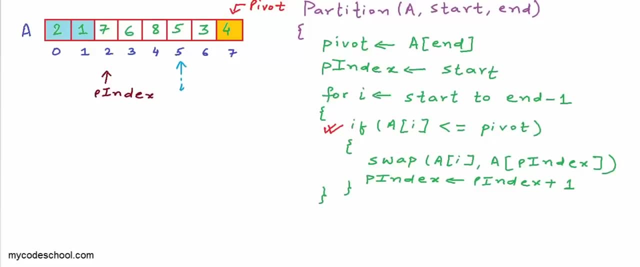 8, once again, is greater than 4.. i will now be 5 and 5.. The element at index 5 is also greater than 4.. So we will go to index 6.. 3 is lesser than 4. So we need a swap here. 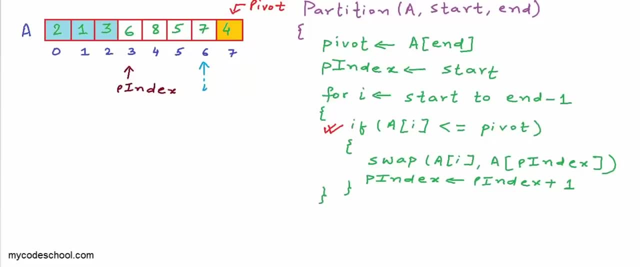 And now p index at this stage will be 3.. And now we will exit the for loop And, if you can see, at this stage all the elements lesser than the pivot are towards the left of the partition index And the pivot itself, and the elements greater than the pivot are. 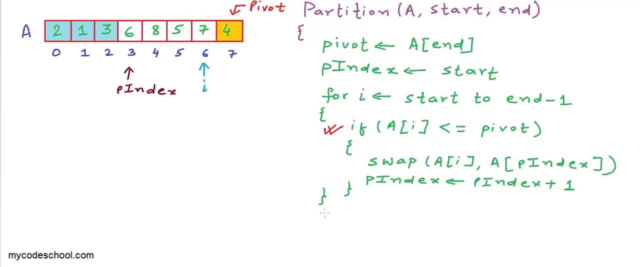 on or after the partition index. Now there is only one more thing that we need to do And we will have a proper partitioning. We will swap the element at the partition index with the element at end index, which is the pivot. So 6 will go to index 7 and 4 will come to index 3.. 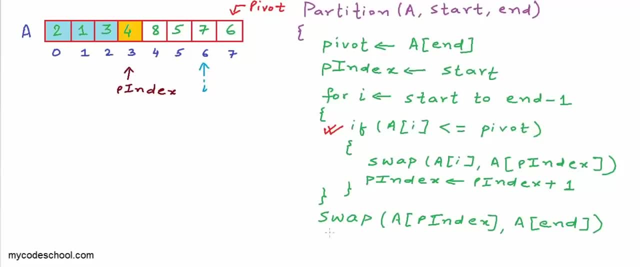 And now we have a proper partitioning This function. partition will return the partition index And we are good With this implementation of partition function. the quick sort function that we had written earlier will work. Let's quickly write a real program for this and see whether this works or not. 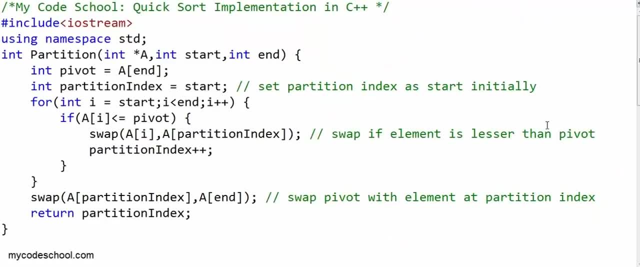 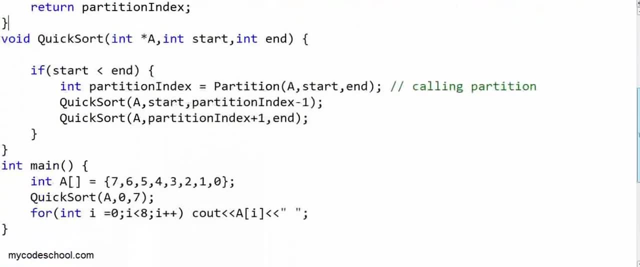 I'm writing this program in C++. This is the implementation of partition function, And then I have written the quick sort function. Inside the quick sort function we make a call to partition and then we make two recursive calls In the main function I have initialized. 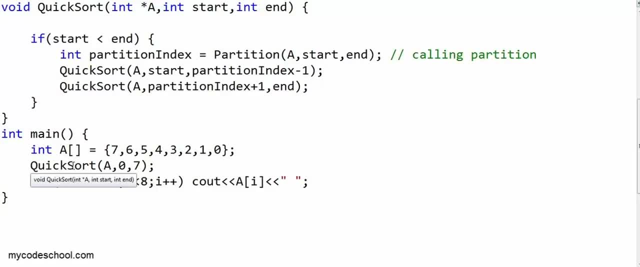 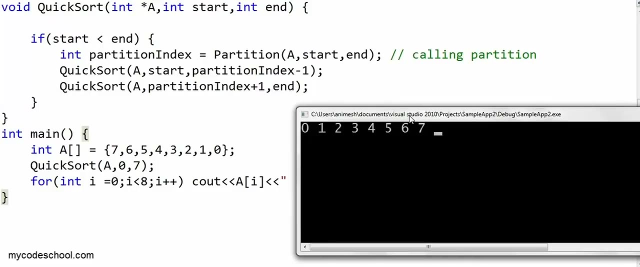 an array of eight elements, then I'm making a call to quick sort, passing starting index zero and index seven, And then I'm simply printing the elements in the array after call to quick sort. Let's see what happens when we run this code. The output seems to be sorted. 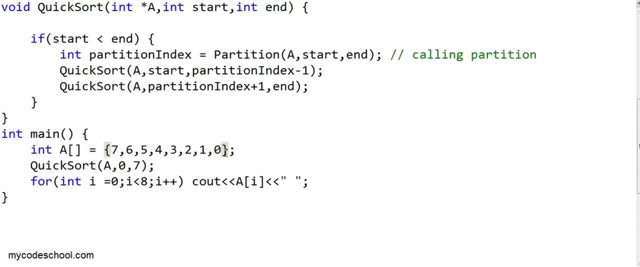 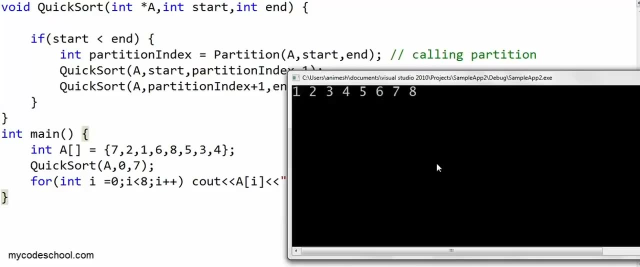 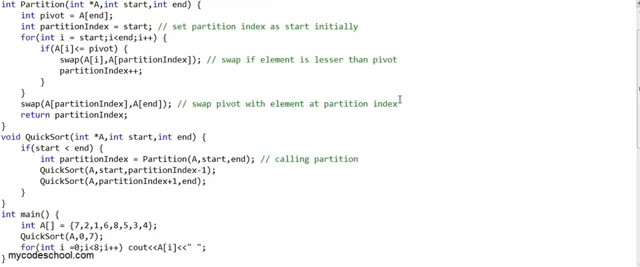 Now let's change this array. Let's pick up, pick up the example that we had used earlier. This is the array that we had used in our example. Once again, the output seems to be correct. So we are looking good. So this is our implementation of quick sort in C++. We 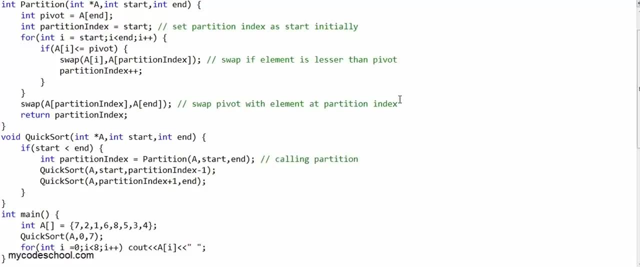 have left one question unanswered. The question was: why are we not having to create an auxiliary array here like merge sort? Well, in merge sort, once we were done sorting the left part and the right part, then we were merging the two parts back into the original list And 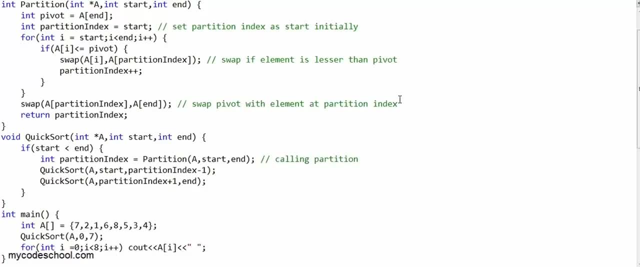 there is no way you can perform the merge process without using auxiliary arrays. Think about it and you should be able to get it. We will analyze the properties and running time of quick sort In next lesson. this is it for this lesson. Thanks for watching. 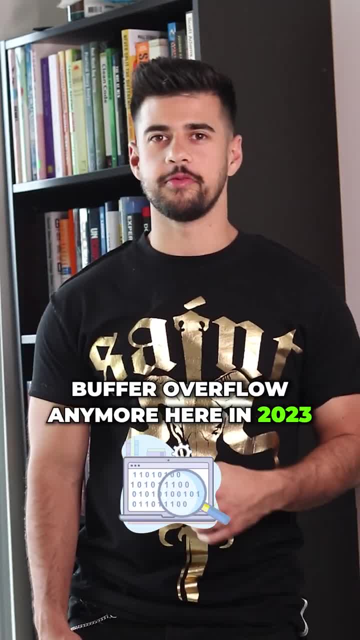 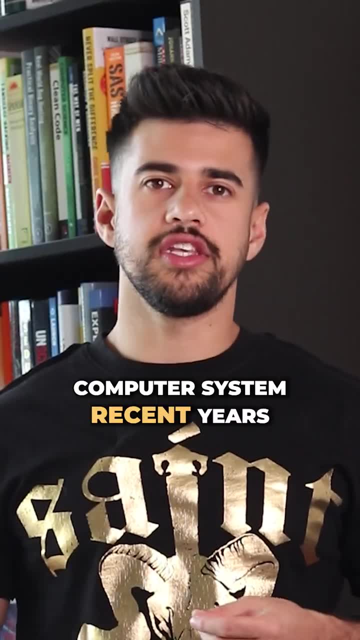 Is it even worth it to learn buffer overflow anymore here in 2023?? If you're not familiar, buffer overflow is generally regarded as a super ancient technique of exploiting computer systems. In recent years, there's just been so many mitigations that have been added, both on the 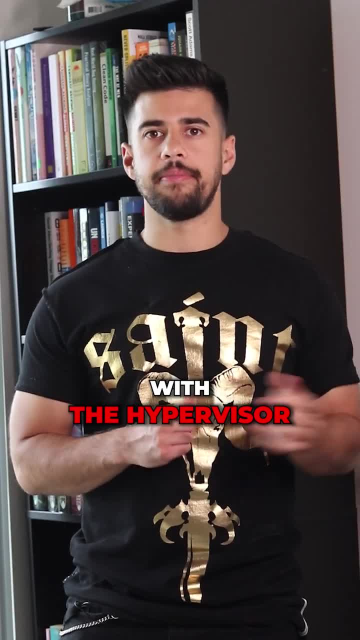 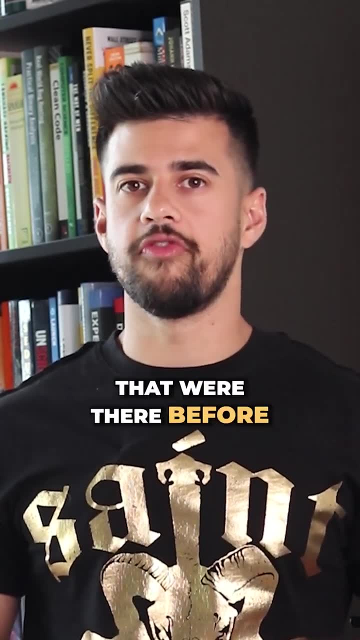 Windows and Linux side. Windows has added HVCI with a hypervisor-based virtualization And heck, the Linux kernel is moving to Rust. that is completely eliminating a lot of the bugs that were there before. Suffice it to say: if you want to exploit a modern system, it's extremely. 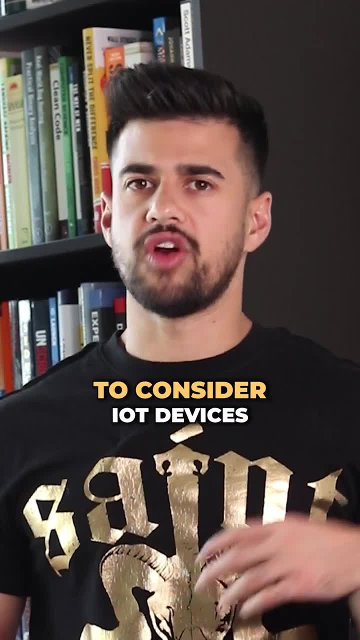 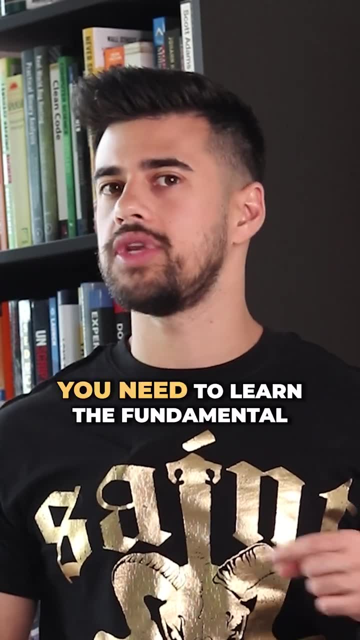 extremely complex compared to what it was back in the day. Here's one thing to consider: IoT devices. they're still using this old stuff And some of those are still vulnerable to your classic buffer overflows. But I would say absolutely. you need to learn the fundamentals to get into.